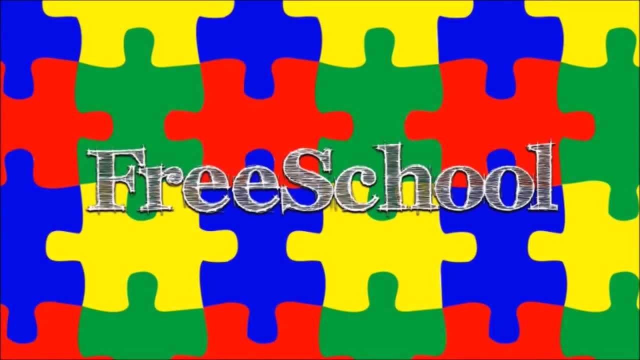 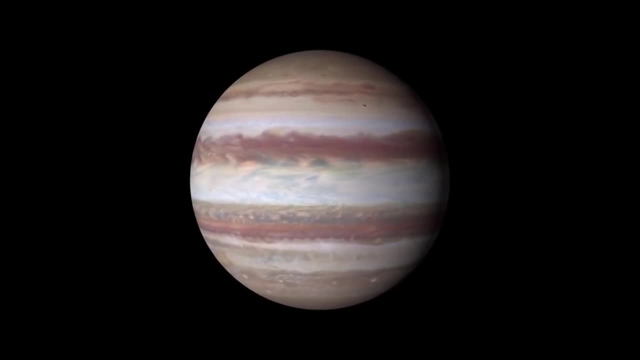 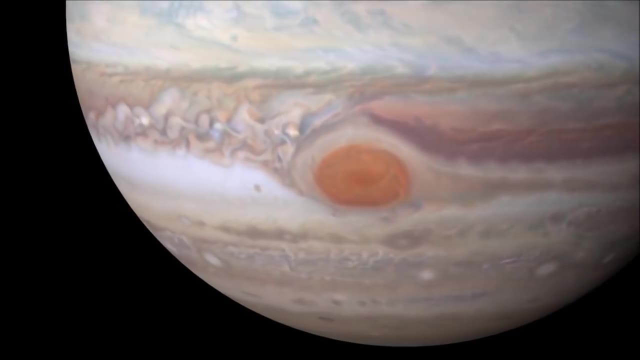 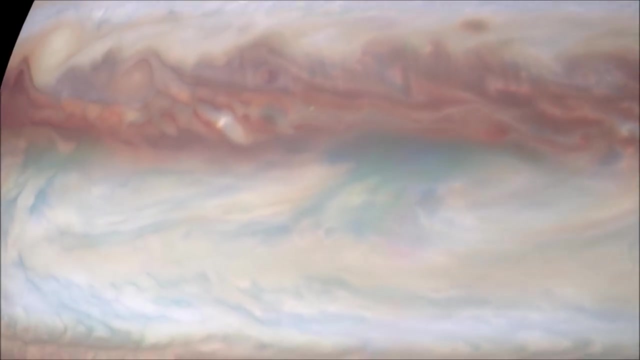 JUPITER, THE FIFTH PLANET FROM THE SUN, IS ALSO THE LARGEST PLANET Aside from the Sun. Jupiter is the largest object in the Solar System. It is called a gas giant because it is so large and it is made mostly of gases- hydrogen. 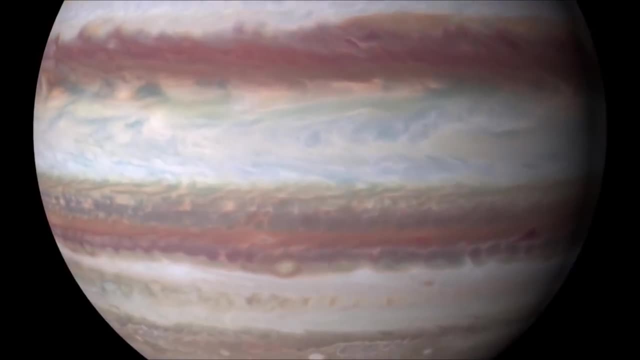 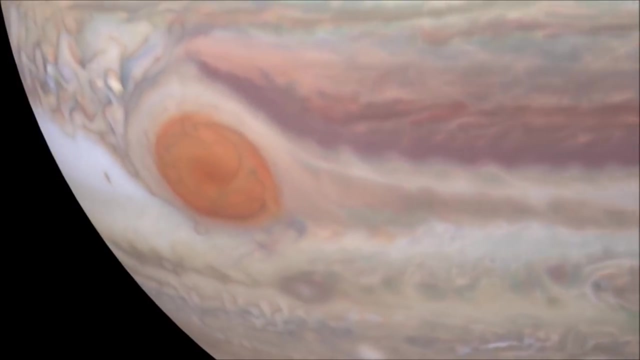 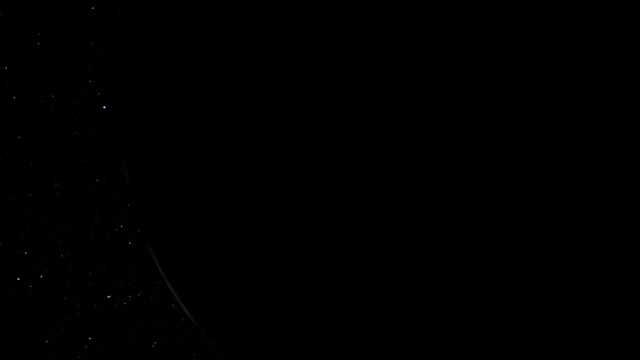 helium, methane and ammonia. Jupiter is made of many of the same materials as stars. If it had been about 80 times more massive than it is, it might have become a star instead of a planet. It would take more than 300 Earths to equal Jupiter's mass. It is twice as massive as 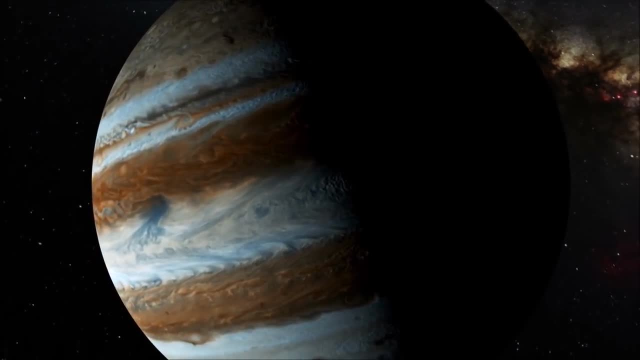 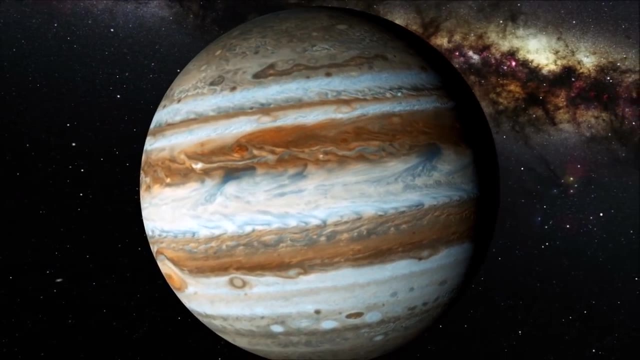 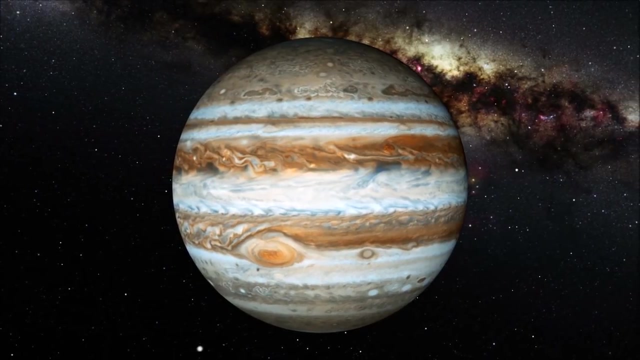 all of the other planets in the Solar System put together, and has a diameter of more than 88,000 miles or 142,000 kilometers. It is so large that, if it were a big jar, more than 1,300 Earths could fit inside of. 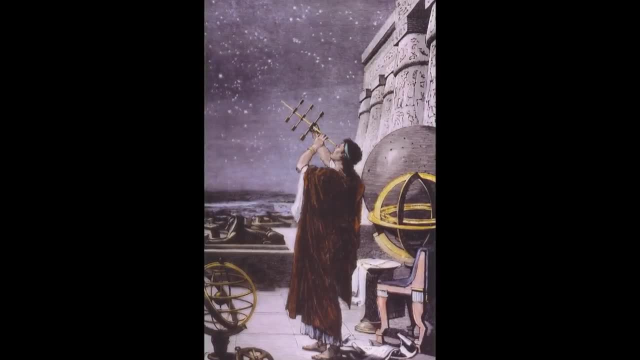 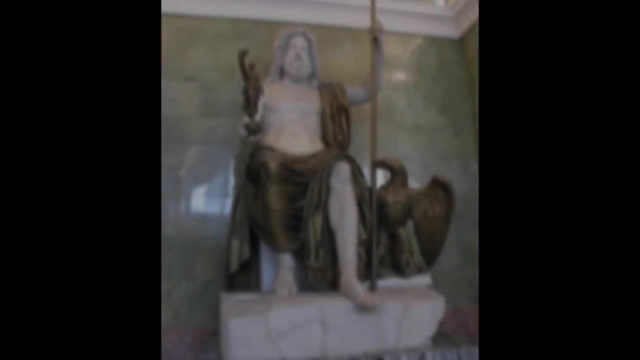 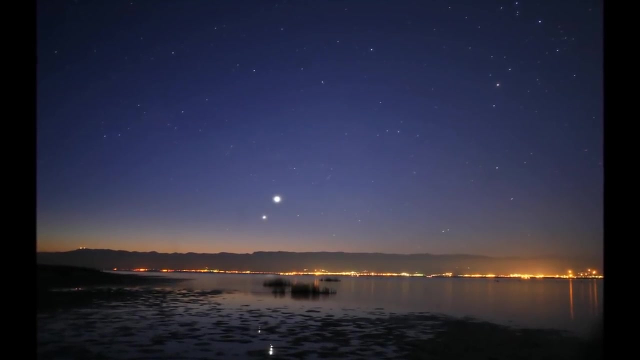 it. Jupiter has been observed for thousands of years and was known to the ancient Romans, who named it after Jupiter, the king of the gods. It is the third brightest object in the night sky. It is the largest star in the solar system, with a diameter of about 25,000 kilometers. 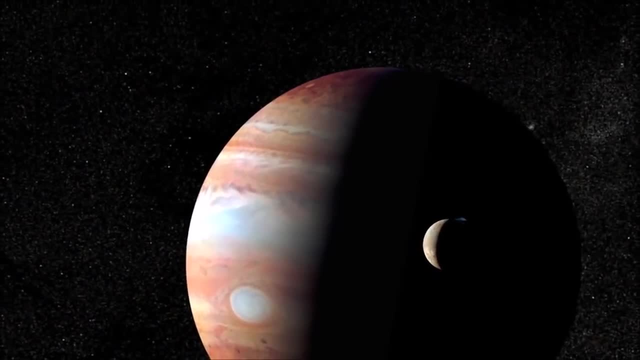 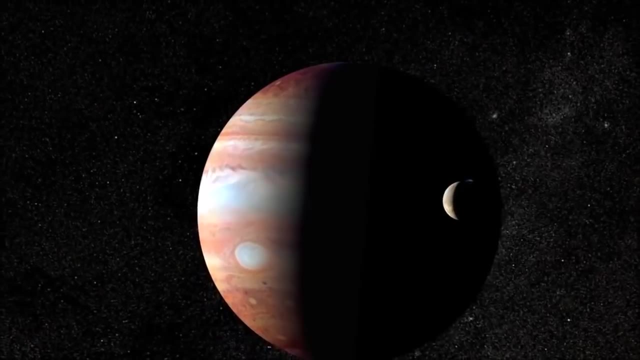 It is the second brightest star in the solar system. with a diameter of about 5,000 kilometers, It is the largest star in the entire Earth. Its orbit is much shorter than that of a moon, dimmer only than the moon and Venus. 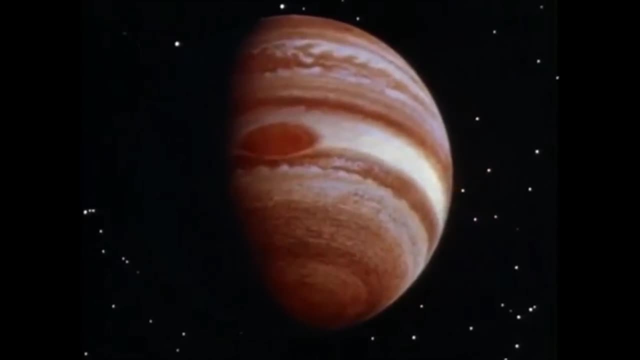 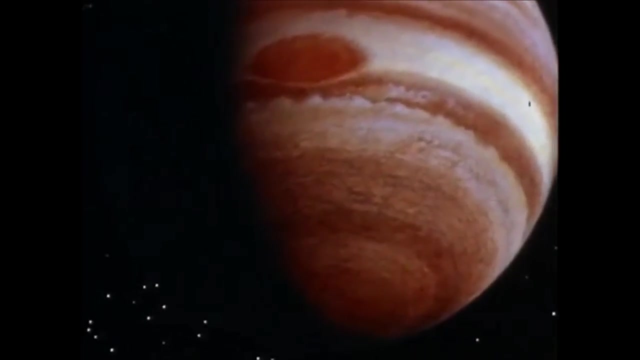 Jupiter is so far from the Sun that it takes more than 11 Earth years for it to travel around once. Although Jupiter's orbit is much longer than the Earth's, its day is much shorter, rotates once about every nine hours faster than any other planet Spinning so quickly. 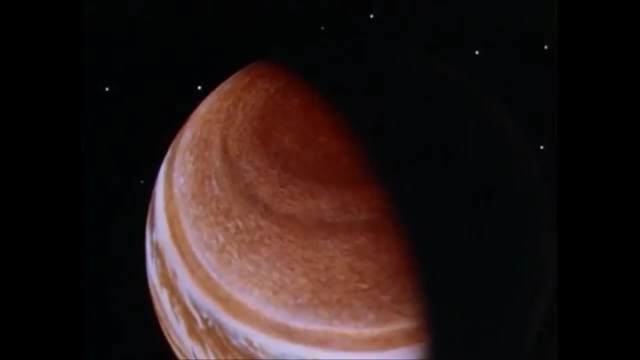 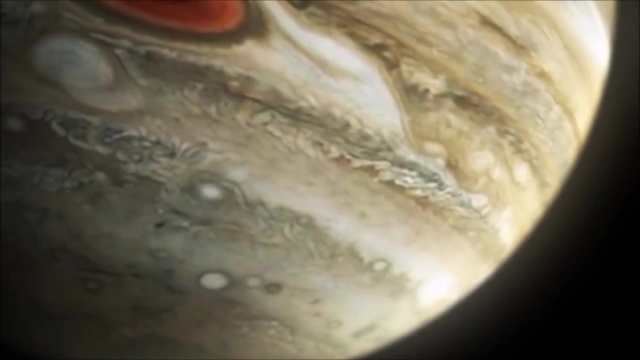 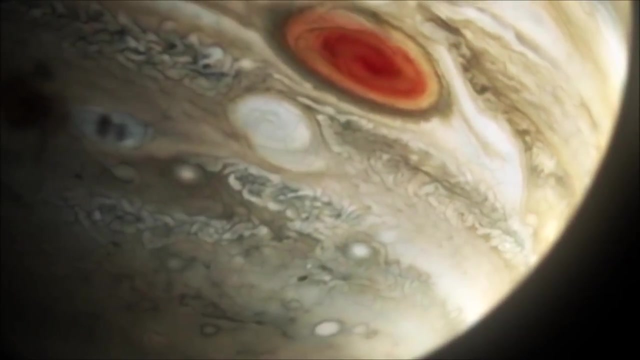 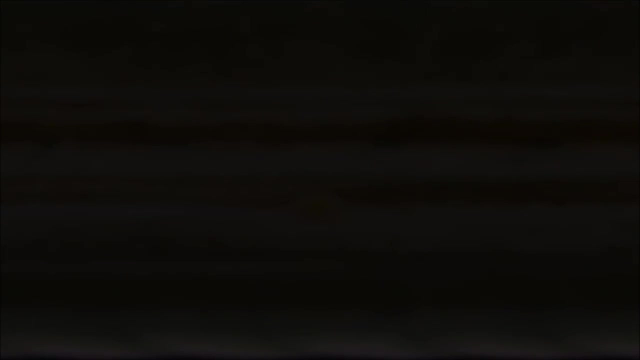 causes strong weather patterns in the clouds surrounding the planet. This makes Jupiter the stormiest planet in the solar system. There is a permanent whirlpool of storms on Jupiter, known as the Great Red Spot, which has been churning for centuries. It was first observed more than 350 years ago by Robert. 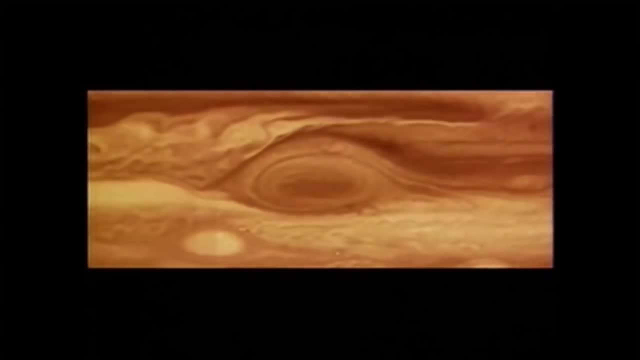 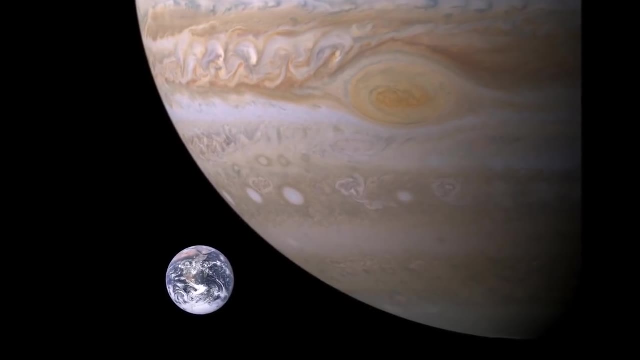 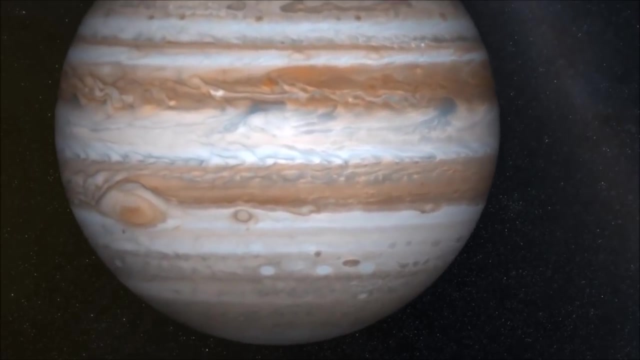 Hooke and can be seen using a telescope. The Great Red Spot is huge. In fact, it is larger than the Earth. However, recent observations have shown that the Great Red Spot is shrinking and is currently at the smallest size it has ever been observed. 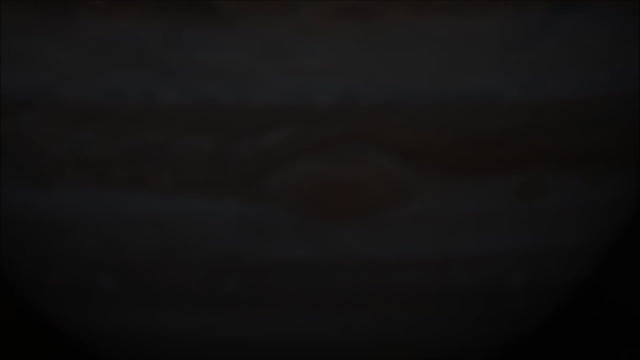 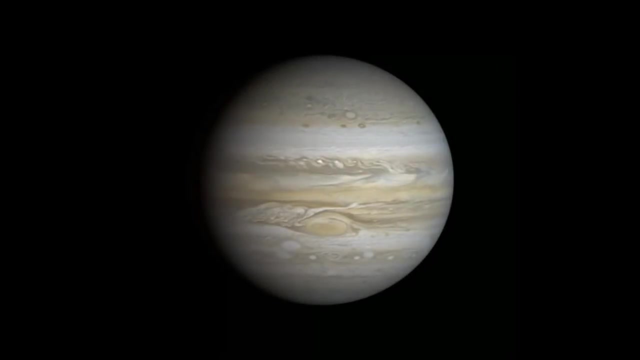 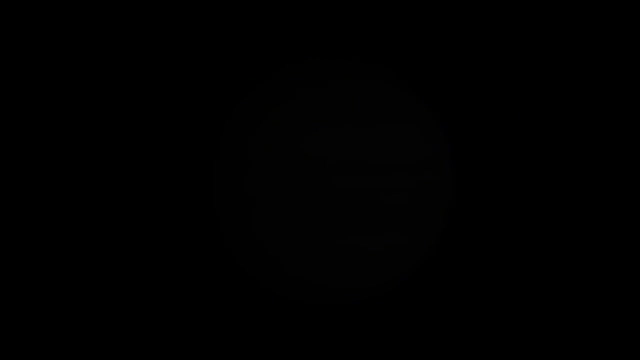 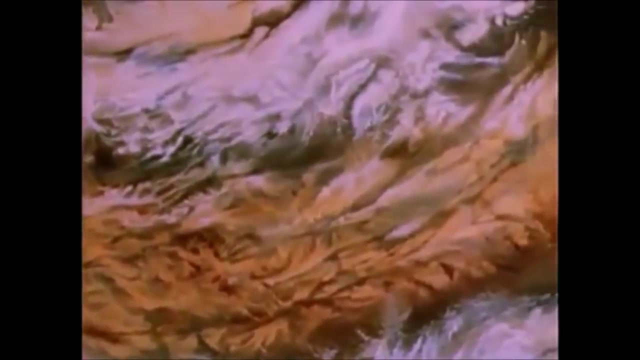 Temperatures in Jupiter's clouds are far below freezing- negative 234 degrees Fahrenheit or negative 145 degrees Celsius. But near the center it is much, much hotter. Core temperatures on Jupiter may reach 43,000 degrees Fahrenheit or 24,000 degrees Celsius hotter. 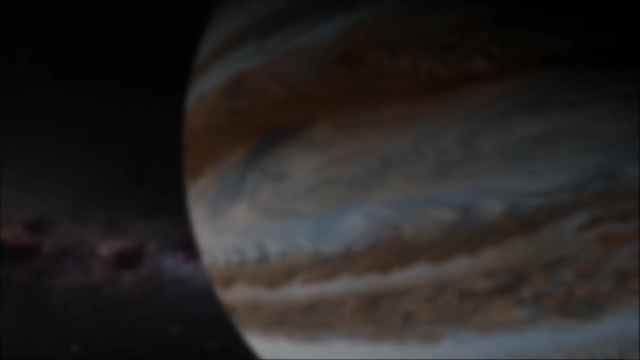 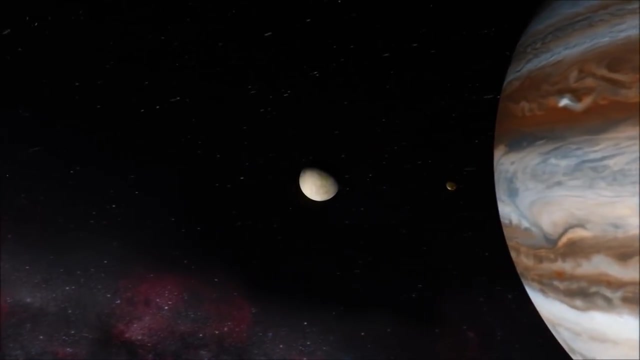 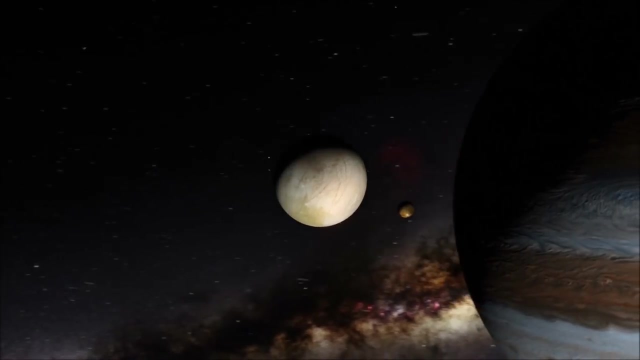 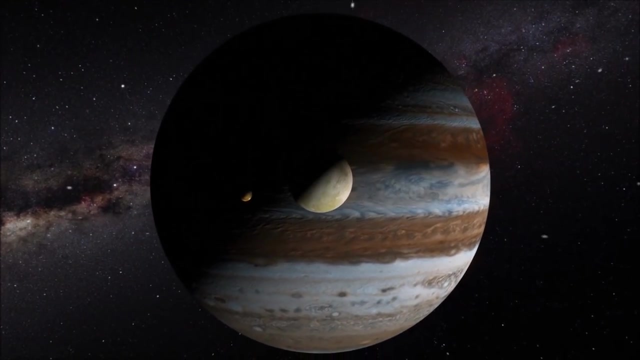 than the surface of the Sun. What Is Supreme Weather? Jupiter has at least 67 moons. 55 of these moons are very small, only a few miles or kilometers wide. The four largest moons, Io, Europa, Ganymede and Callisto, are large enough to be seen. 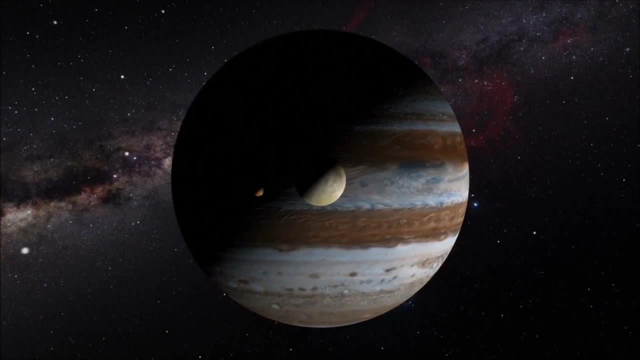 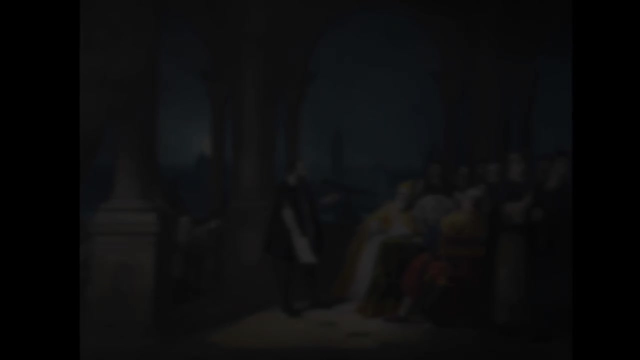 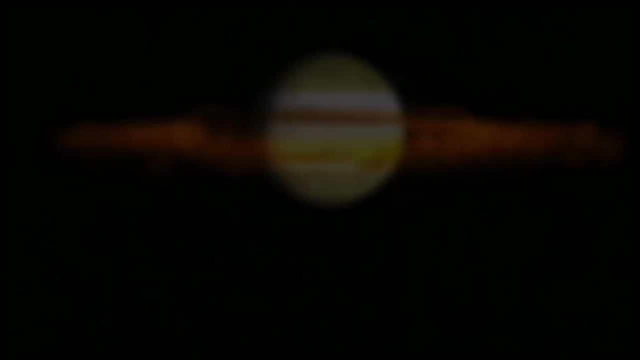 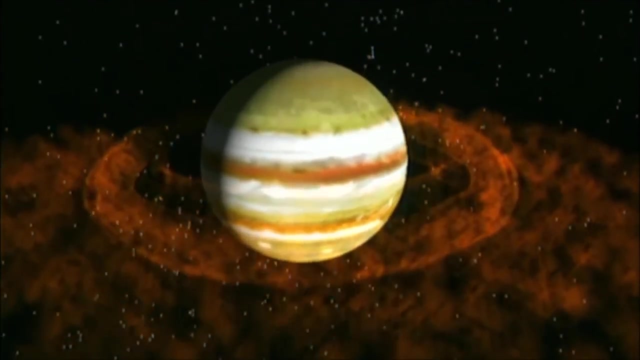 from Earth with a telescope. They were discovered by the Italian astronomer Galileo Galilei about 400 years ago ago. Ganymede is the largest moon in the solar system and is even larger than the planet Mercury. Jupiter also has a system of thin rings around it, although these rings are much, much smaller. 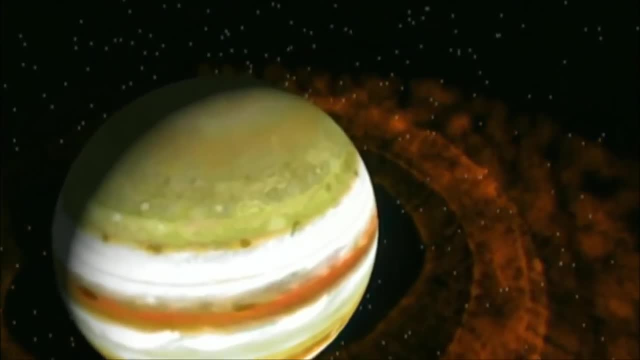 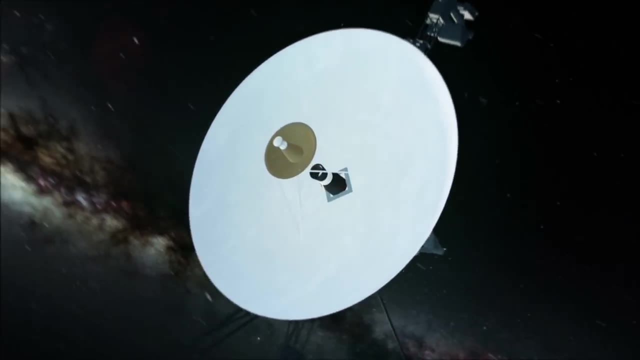 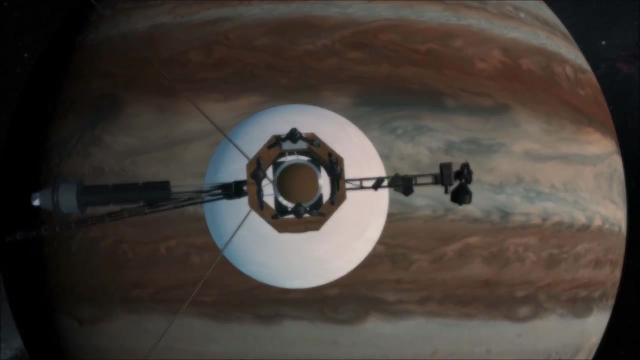 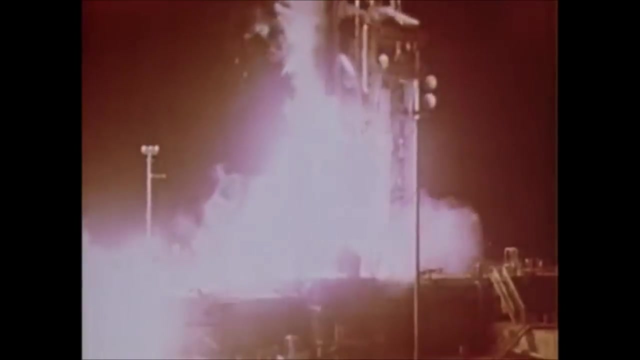 than Saturn's. Made mostly of tiny dust particles, they are so thin and so hard to see that no one knew they were there until NASA's Voyager 1 probe approached Jupiter in 1979.. Eight spacecraft have either passed or visited Jupiter since 1973.. On August 5th 2011,, NASA.